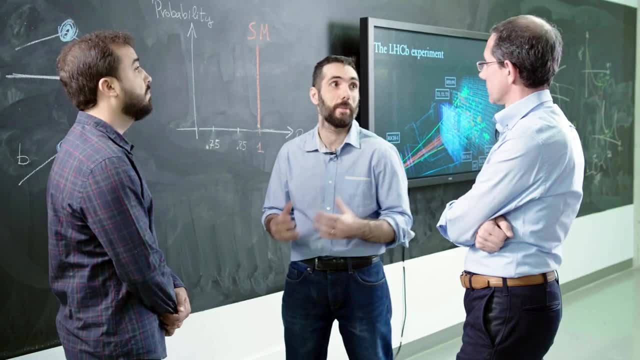 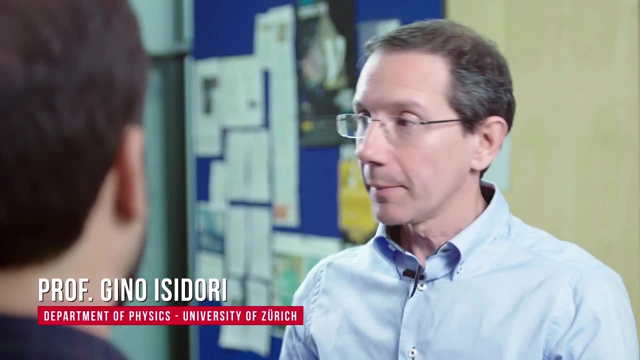 This starts to become pessimistic about the fact that this could be a real breakthrough in particle physics. I don't agree. I don't share this pessimism. It's true that this result is inconclusive, but I don't think there is any reason to be more pessimistic than we were before this measurement. 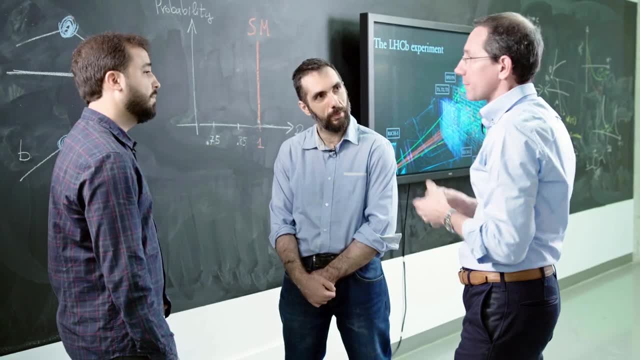 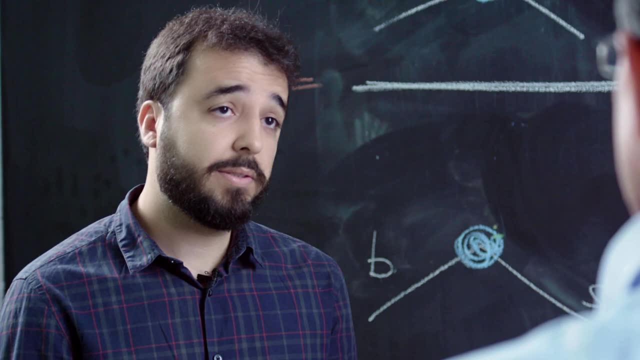 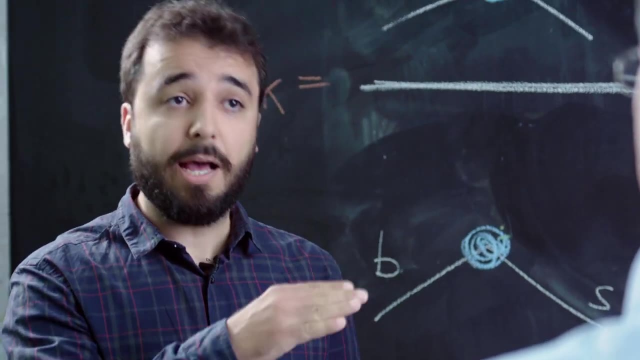 The probability of a discovery is exactly the same that we had before. I'm stunned by how emotional is our community In the end. this is exactly how particle physics works. Some discoveries are very rare. They usually have small deviations or evidence that start to pile up with time. 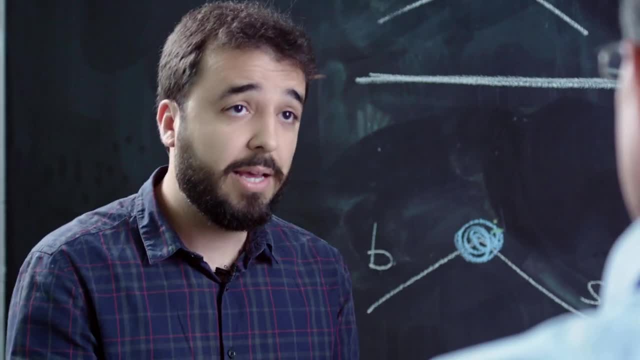 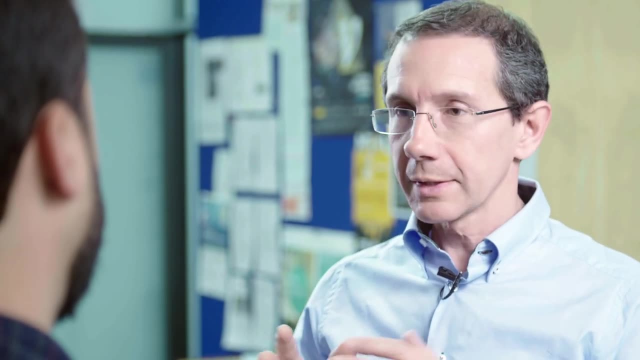 that suddenly, at some point, will converge into the real facts, And I think we might be actually in the exact situation that we are facing now. Okay, so let's try to understand what happened. We have the standard model, as you know, this beautiful theory that describes very well. 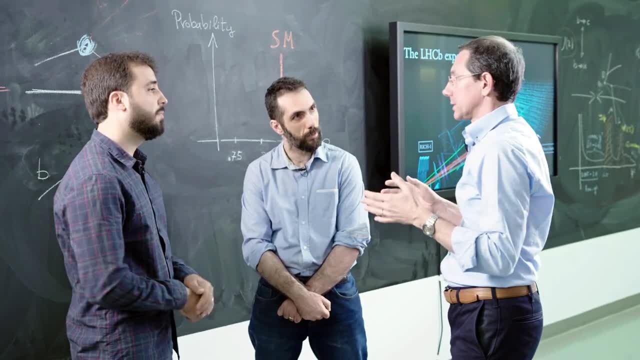 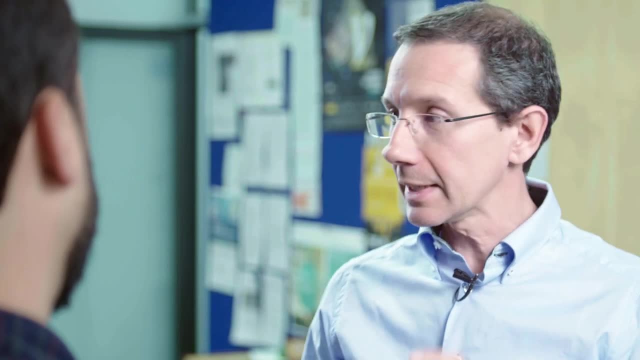 the nature of the elementary particle and the forces through which they interact. And we know that this theory works very well. It has been tested by thousands of experiments. but we also know that this theory is incomplete. In particular, it doesn't tell us why different particles have different masses. 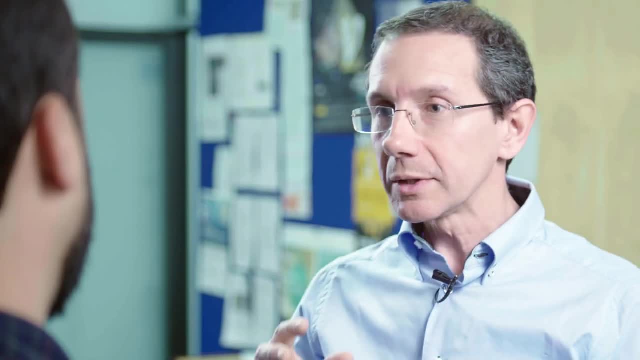 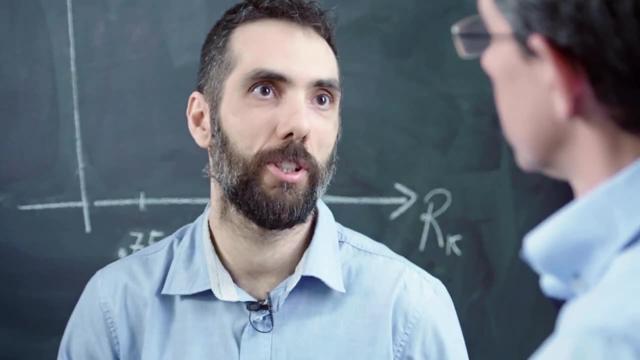 These anomalies observed by the LACB could be the first hint of a new interaction that could explain, address this fundamental question. And indeed we do have two anomalies, Gino. The one we are considering now consists of a B quark decaying into an S quark and a pair of other particles. 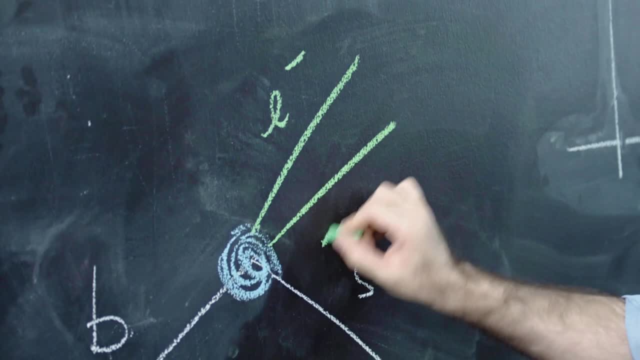 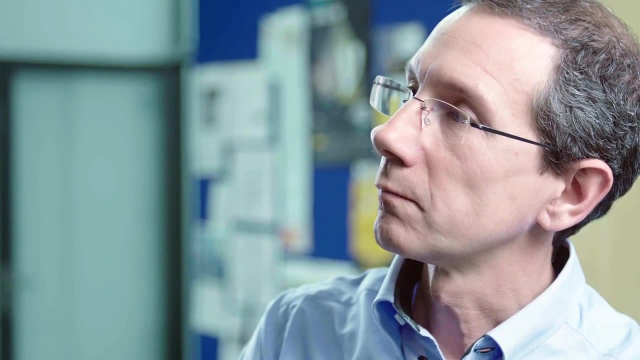 In particular, an electron and an anti-electron, And a muon and an anti-muon. The standard model, as you said, has a very clear prediction. It predicts that the frequency of this process and this process is the same. 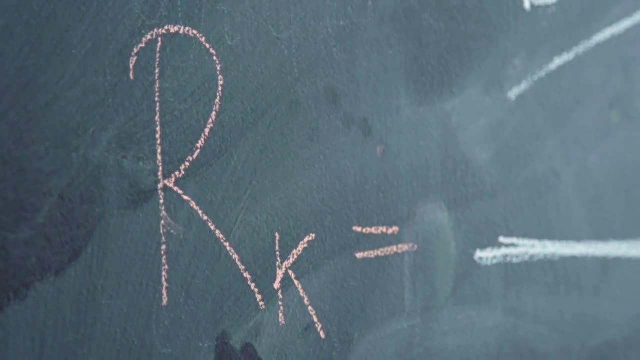 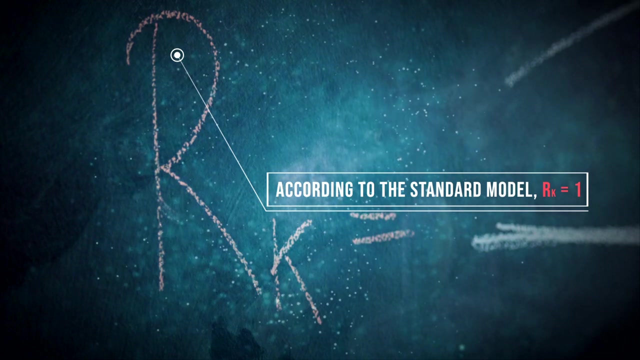 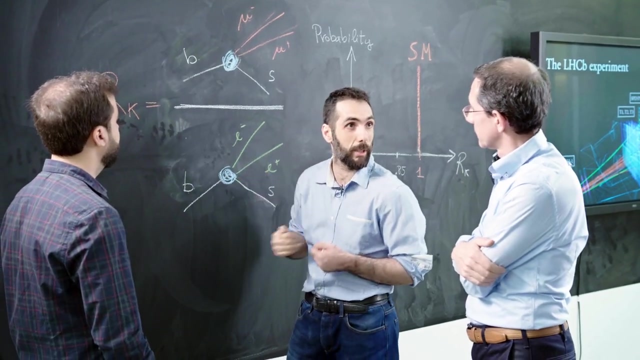 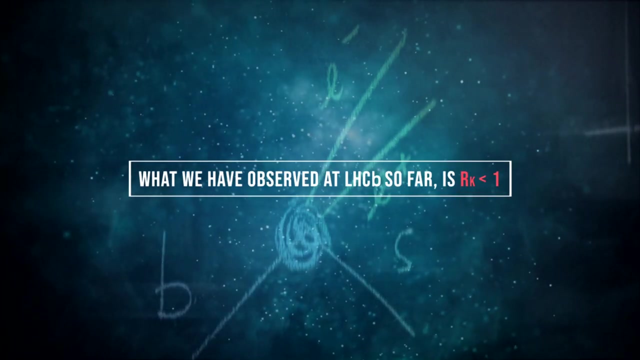 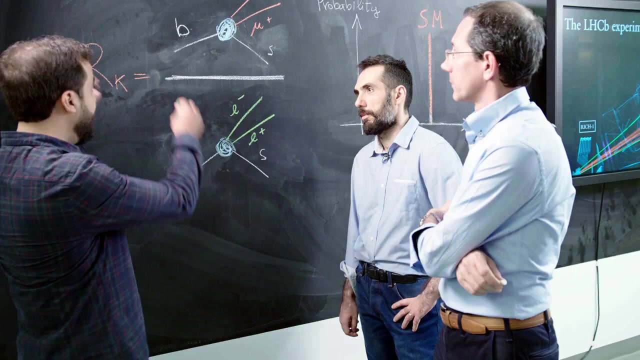 Therefore, this ratio that we call RK should be one. What we have observed in LACB is a deficit of muons with respect to electrons. Therefore, this ratio appears to be smaller than one, And the best way to visualize this is putting a probability plot. 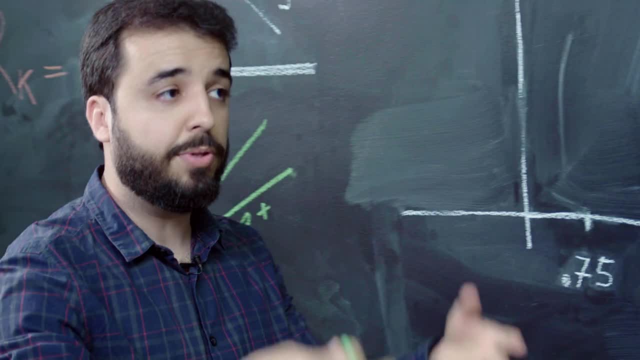 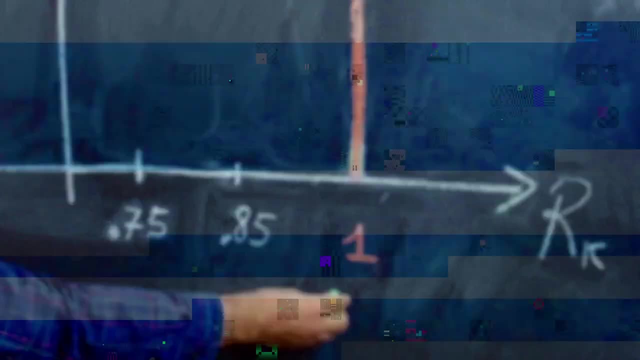 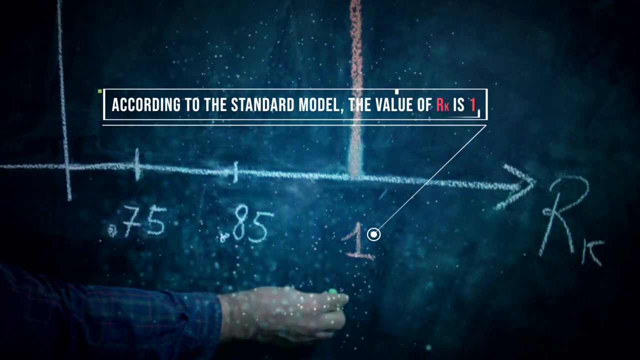 What we have here are different values of RK, so the ratio between muons over electrons as a function of the probability. So in the standard model you expect this to be precise at one. However, as Nico pointed out, the first measure of LACB- 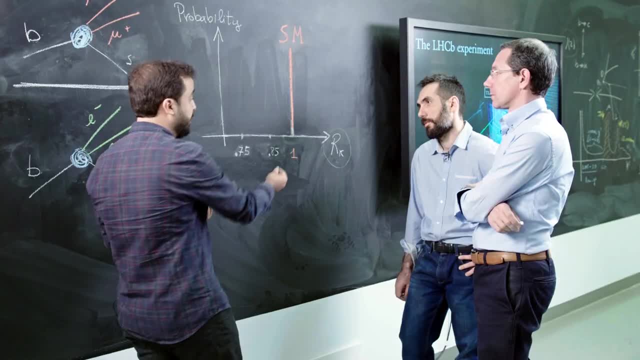 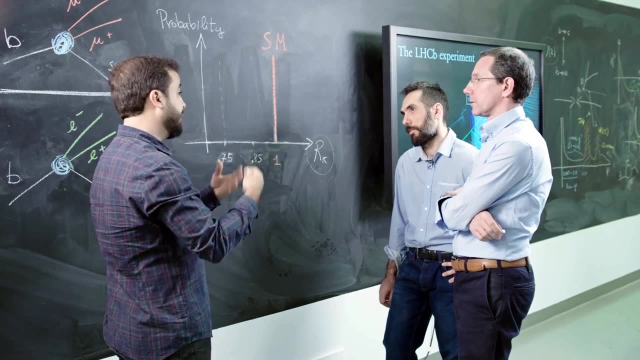 was actually showing a deficit of muons over electrons And therefore it pushed the value to be below one To this value here. But when we actually perform measurements we have associated to it some uncertainties. So the best way to see this here would be in this kind of probability curve. 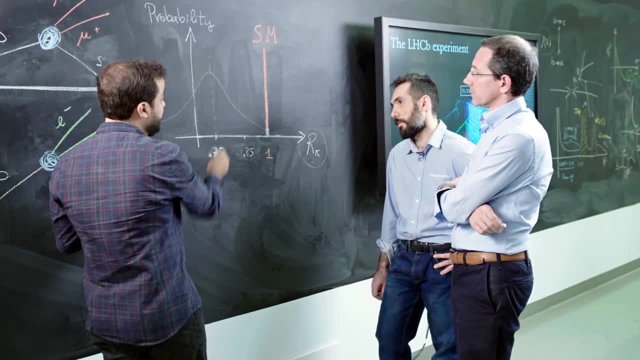 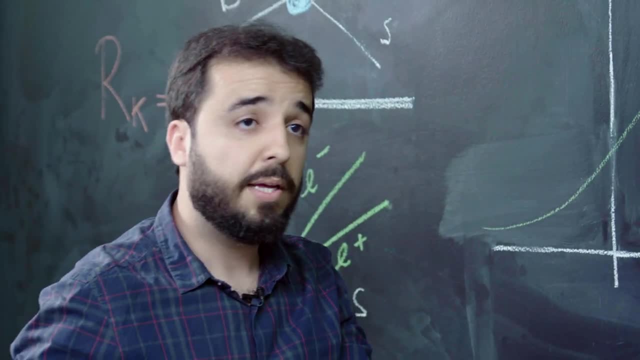 And the value that you can see here on the top is just the most probable value still, but there is still some chance that this is to be compatible with the standard model. This is about 2-3% And in order to go further and make a claim of this cover: 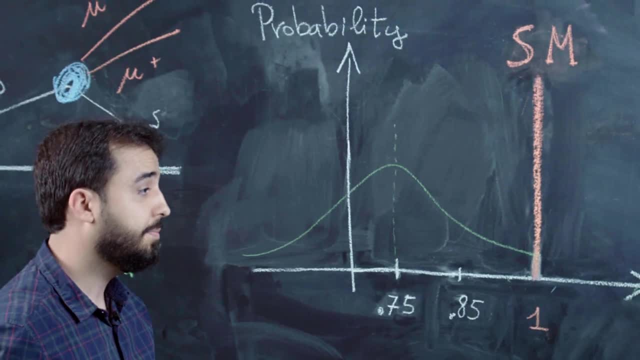 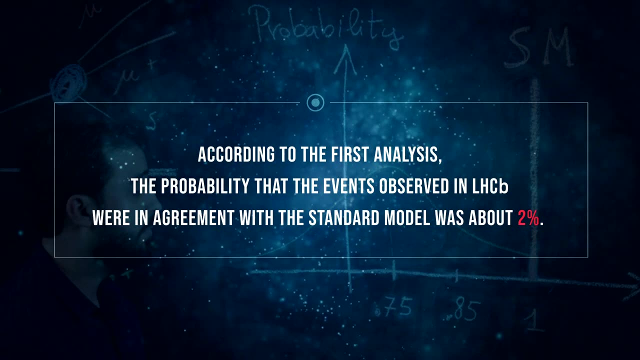 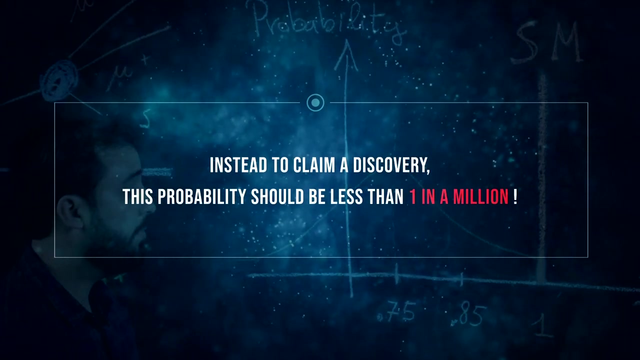 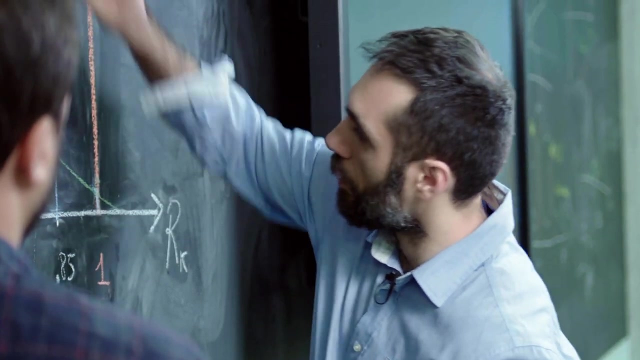 this probability has to be below one in a million. Yes, and the new measurement is around here with a probability curve like so. Therefore, while the uncertainty is reduced, it is also closer to the standard model, And the irony is that this probability is still 2-3%. 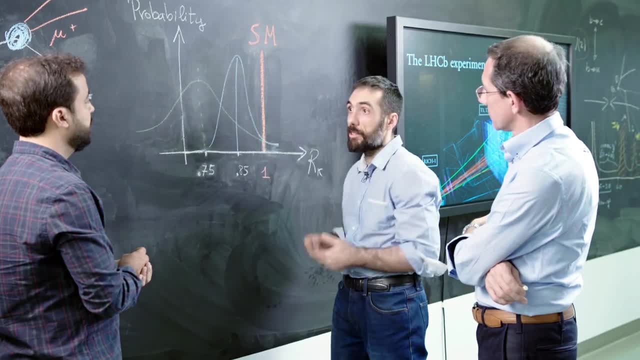 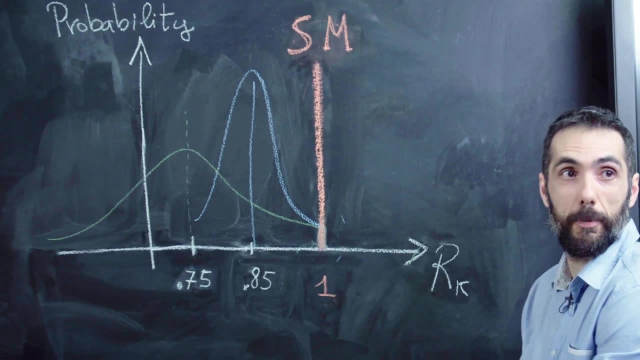 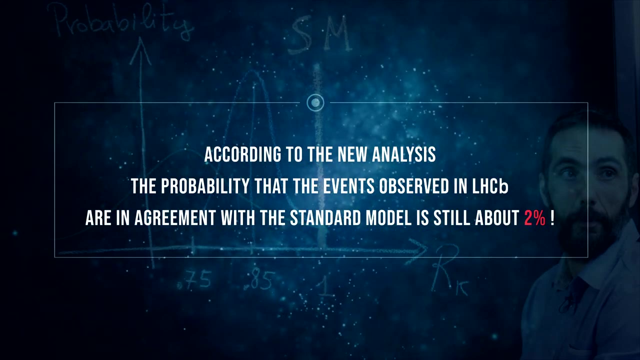 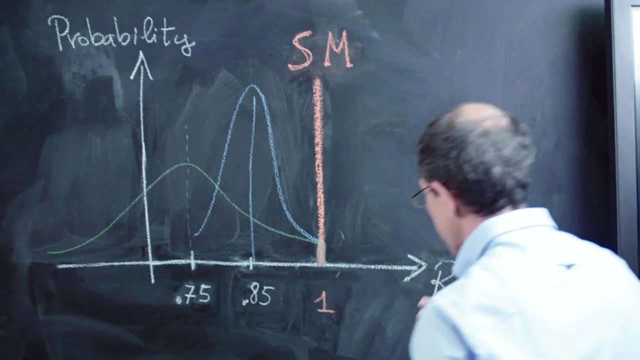 That's why I say that the new measurement is basically inconclusive. unfortunately, This is inconclusive, but I think there is no reason to be more pessimistic than before because, you see, we have to remember that we know very well what is the standard model value. 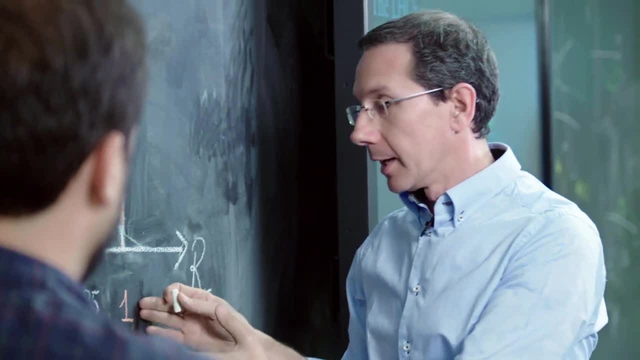 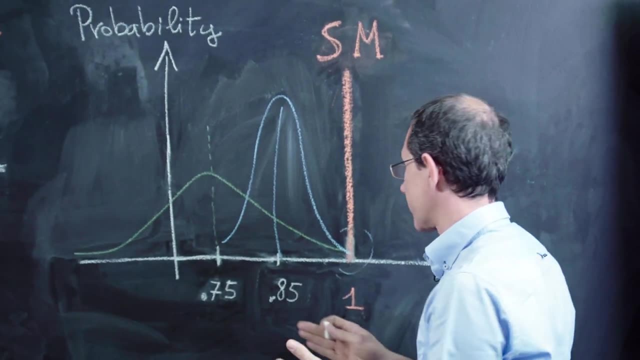 which is one, but we don't know which can be the value beyond the standard model. Any value over here clearly different from one can be explained only by a new force, and this will be a major discovery. This is still highly probable. 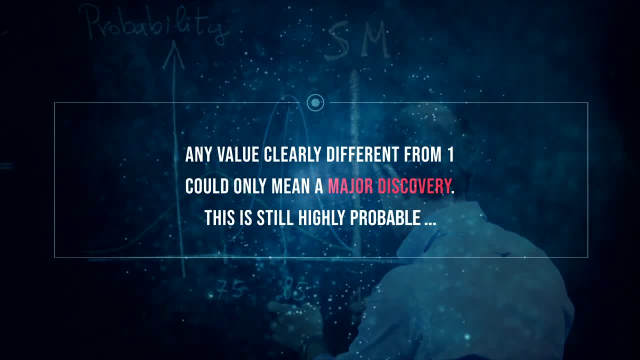 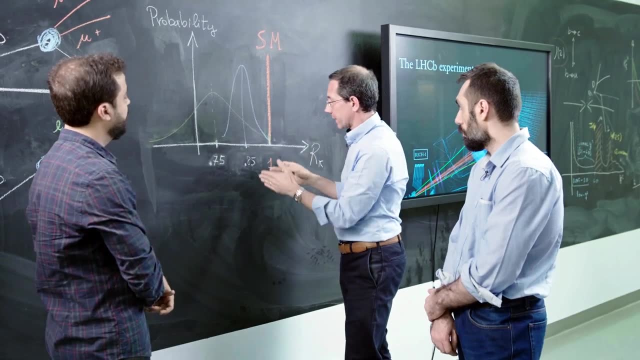 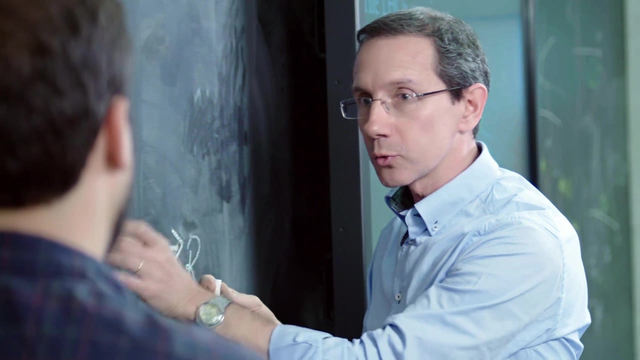 And actually a value like this one here. if the result will have a smaller error, it fits even better with our theoretical model. So I think the solution is still extremely interesting, I mean if the data will converge to this value here.